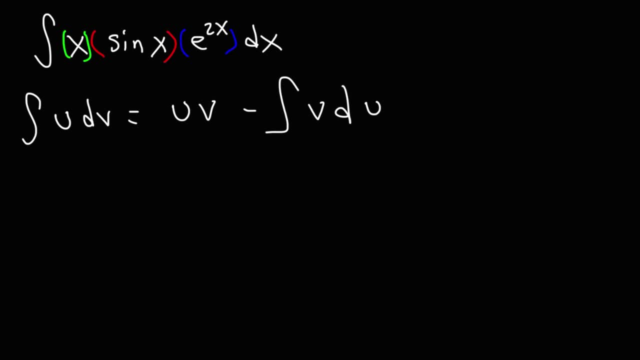 the integral of v du. Now, this works for a two product term expression, but what about a three product term expression? Well, before we can derive the formula that will help us get the answer, let's talk about how we can derive this formula, because, if we can understand that process, 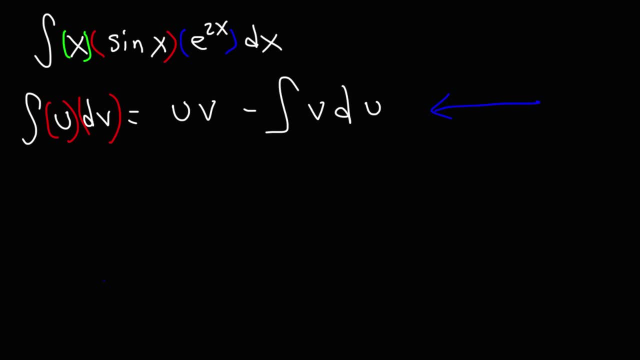 we can apply it to a three product term expression. We need to start with the product rule. The integration by parts is basically a reverse or the reverse process of finding the derivative using the product rule. So let's say we have a two product term expression. 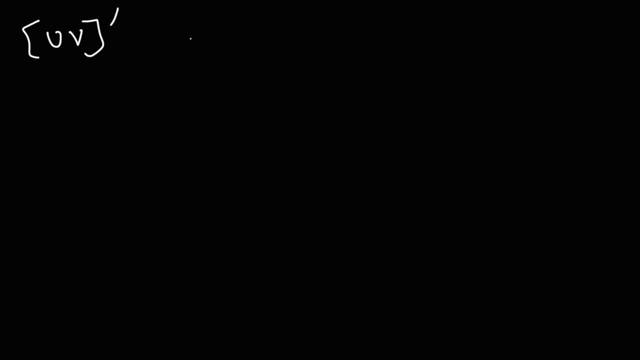 u times v, The derivative of u times v is going to be: you take the derivative of the first part, u, which becomes u prime times v plus u times the derivative of the second part, v prime. So that's the product rule. Now u prime, if we differentiate it with respect to x, is going: 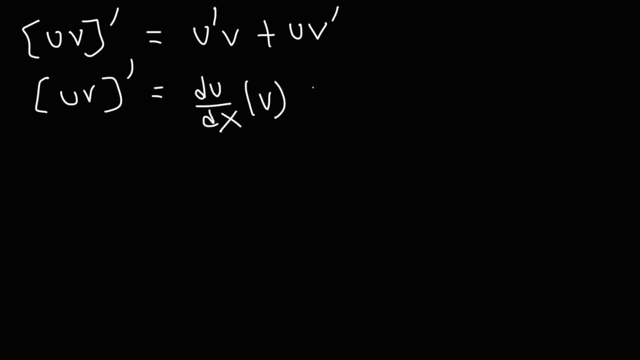 to be du dx and v prime is going to be dv over dx. So what I'm going to do at this point is multiply every term by dx. So I now have u v prime. dx is equal to v du plus u dv. So at this point, what I'm going to do now 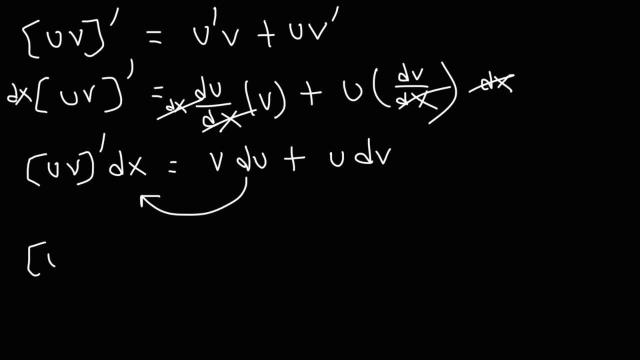 is. I'm going to move this term to the other side. So I have u v prime dx minus v du is equal to u dv. Now I'm going to reverse the equation, I'm going to take this term and I'm going to take this term. 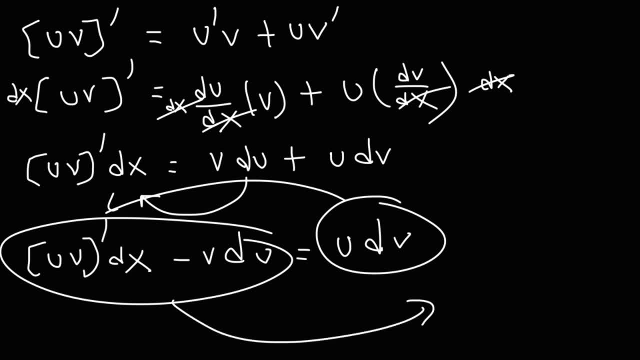 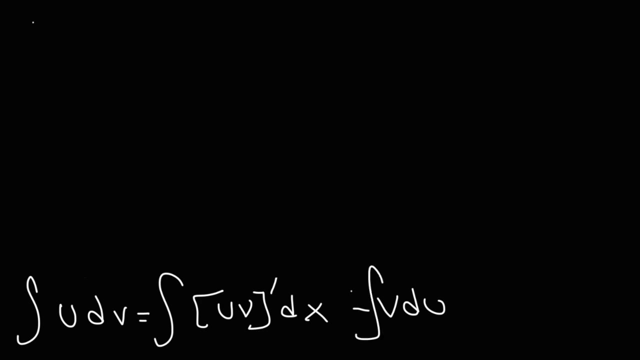 and move it to the other side, and this move it to that side, So reversing the equation. we're basically just switching it. I have u dv is equal to u v prime dx minus v du. So now let's take the integral of both sides, So this becomes the integral of u dv. 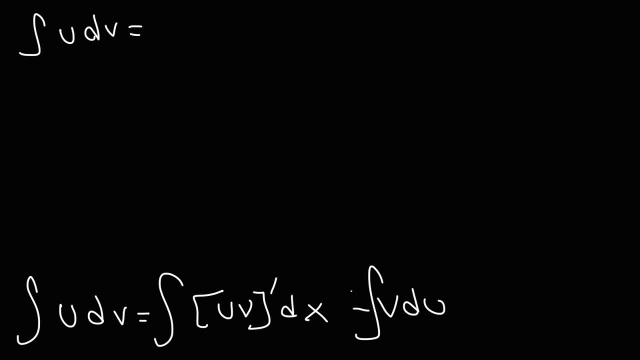 The integral of u v prime is just going to be u v, because here you're taking the derivative and then you're integrating it, which are basically reverse processes of each other, So it's like a double reverse. So you just get u v minus the integral of v du. So that's a simple way in which we can derive the integration by 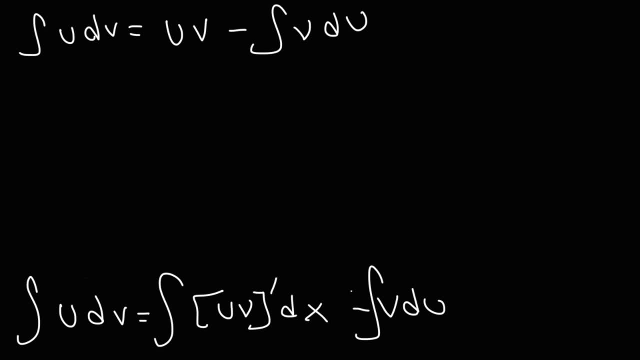 parts formula from the product rule of finding derivatives. Now let's apply that same process to a three product term expression. So let's find the derivative of u, v, w. So first we need to differentiate the first part, So we're going to get u prime, leaving the other. 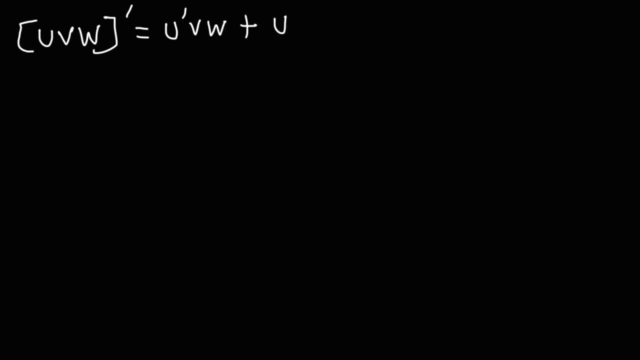 two the same. Next, we need to differentiate the second part, that is v. So that's going to be v prime, leaving u and w the same. And then we're going to differentiate the third part, leaving the first two variables the same. So that's how we could find the derivative of a three product term. 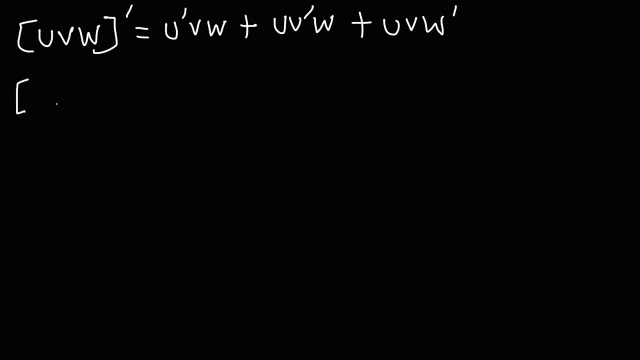 expression. So now, at this point, let's replace u prime with du dx, and we're going to replace v prime with dv dx and w prime with dw dx And, like before, we're going to multiply every term by dx. So these will cancel. 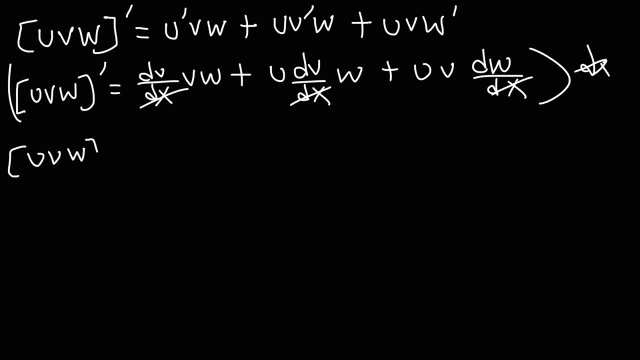 So we're going to get u v w prime times dx and that's gong to equal v w du plus u w dv plus u v dv. Now I'm going to take these two terms and move it to the other side. So I'm going to have u v w prime dx minus v w du, minus u w dv, and that's going to equal u v dw. 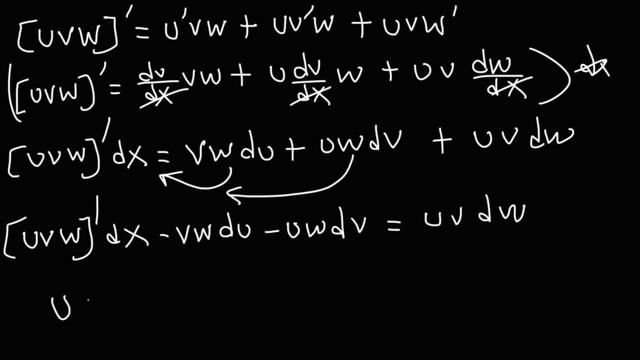 Now I'm going to reverse both equations, So we're going to have: u v dw is equal to u v w prime times, dx minus v w du minus u w dv. Now we're going to integrate every expression or integrate both sides of the equation. 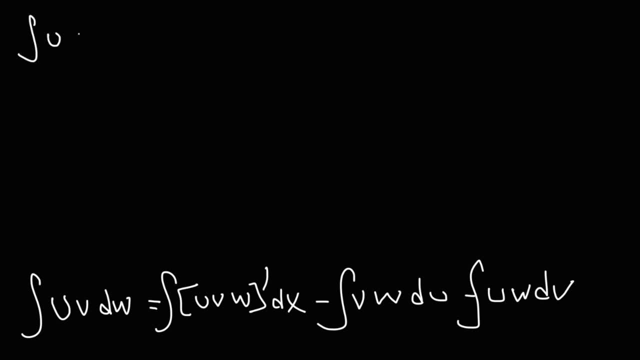 So the final answer is this: The integral of u v dw is going to be: this: becomes just u v w minus the integral of v w du, minus the integral of u w dv. So this is the integration by parts formula for a three product term expression. 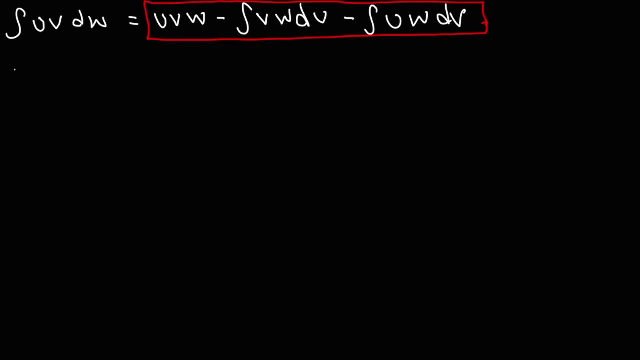 So let's apply this formula to the original problem. So we have the integral of x sine x, e to the 2x dx. So u is going to equal x, v is going to be sine x, dw is going to be e to the 2x dx. 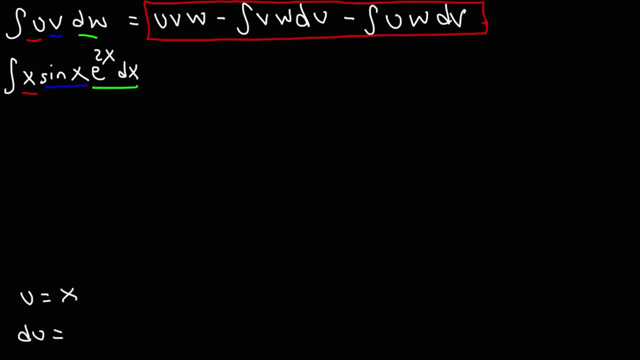 So if u is equal to x, du is going to be the derivative of x which is 1 times dx, Which we can simply write as dx. v is equal to sine x. The derivative of sine x is cosine x, So dv is going to be cosine x dx. 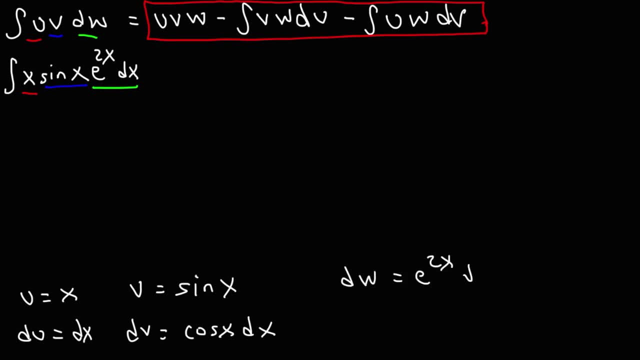 dw is e to the 2x dx. The antiderivative of e to the 2x is going to be e to the 2x divided by 2.. The derivative of 2x is 2.. So now this is going to be u, v, w. 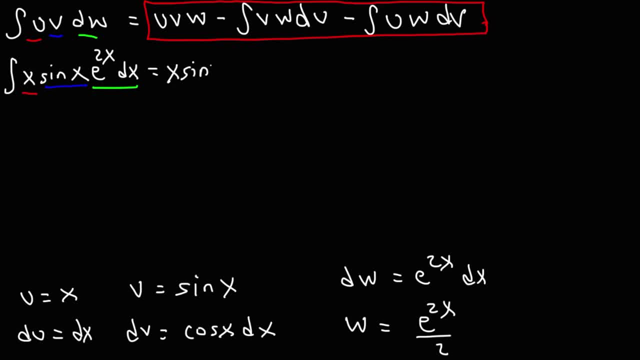 So that's x sine x Times, w, which is e to the 2x over 2.. Minus the integral of v, which is sine Times, w which is e to the 2x over 2.. 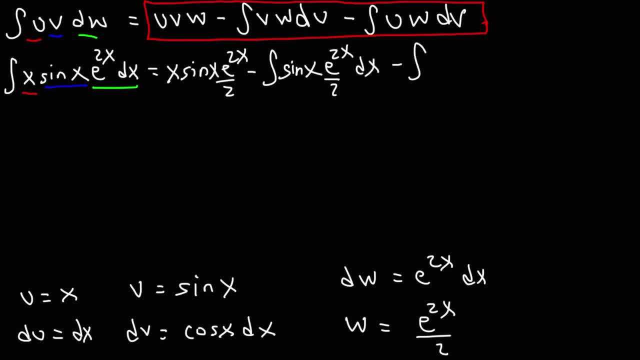 Times dv, which is dx, Minus the integral of u, which is x Times w Times dv, dv is cosine x, dx. So we have a lot of integrals to deal with here, But what we're going to do 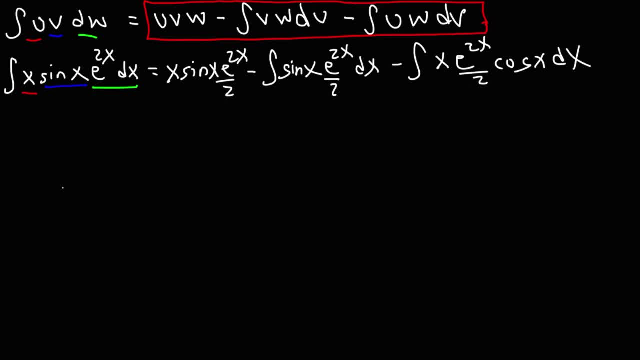 What we're going to do now is we're going to focus on this integral that we see here. So that is 1 half the integral. I took the 2 and moved it to the front, So there's the 1 half symbol. 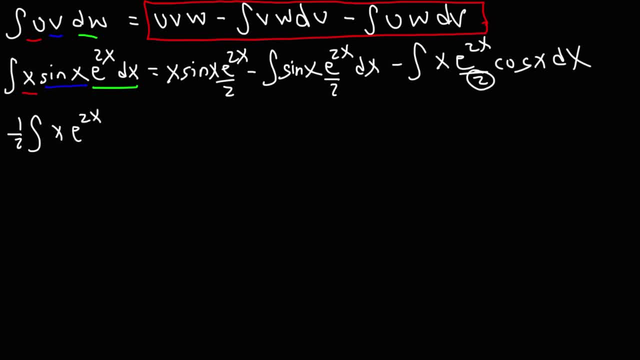 1, half the integral x e to the 2x cosine x, dx. Now we need to use this formula again. So we're going to make u equal to x, So du is dx again, And let me rewrite it. 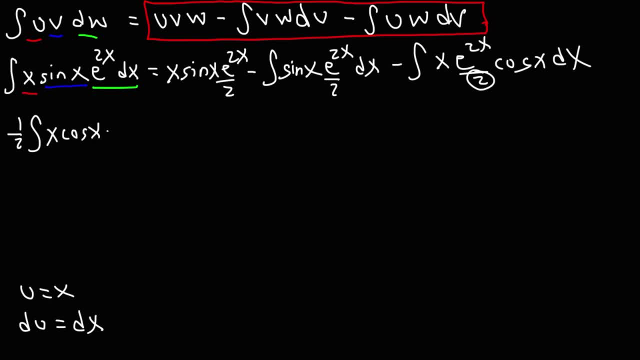 I'm going to write it as: x, cosine, x, e to the 2x, So v is going to be cosine. The derivative of cosine is negative sine, And then dw is e to the 2x dx, So w is going to be the same thing. 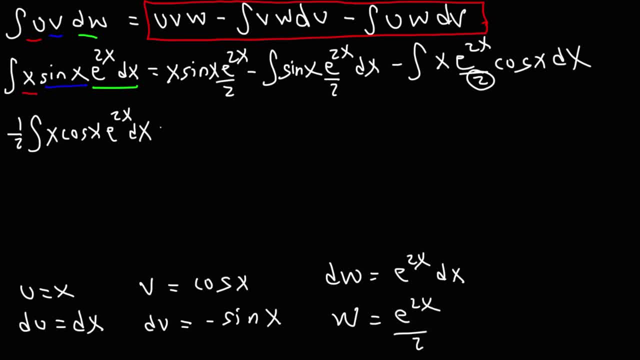 e to the 2x divided by 2.. So now let's put it together. So we have uvw, that's x cosine x, e to the 2x over 2, minus the integral of vwdu. 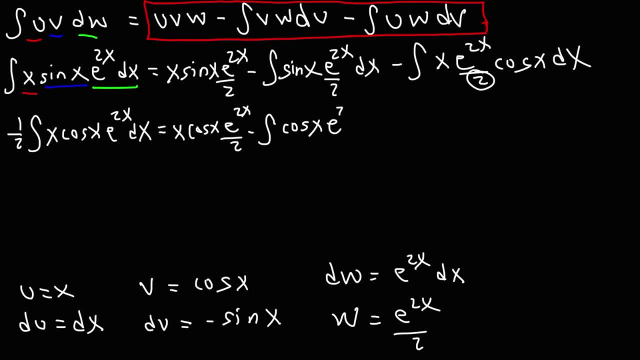 v is cosine, w is e to the 2x over 2.. And du is dx. And then minus the integral of uwdv, u is x, w is e to the 2x over 2.. And du is dx. 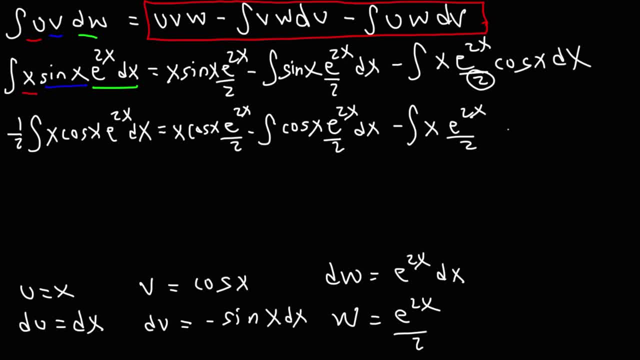 And dv is negative, sine x, dx. So notice that this expression is similar to the original one. So therefore we can combine those two integrals later. So we just need to worry about this one. But now let's move on and deal with this integral. 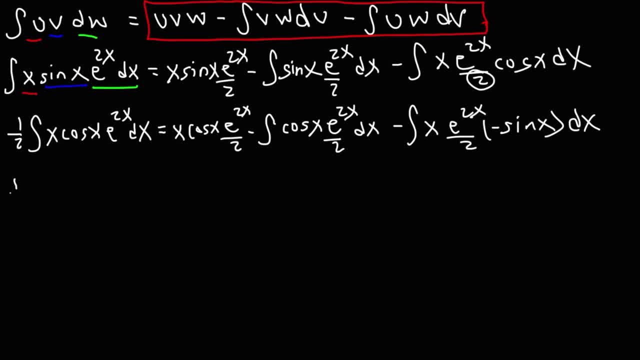 It's a two-product term expression. So we're going to have 1 half, 1 half And that's the integral of sine x, e to the 2x. So we're going to use this formula: The integral of udv is equal to uv minus the integral of vdu. 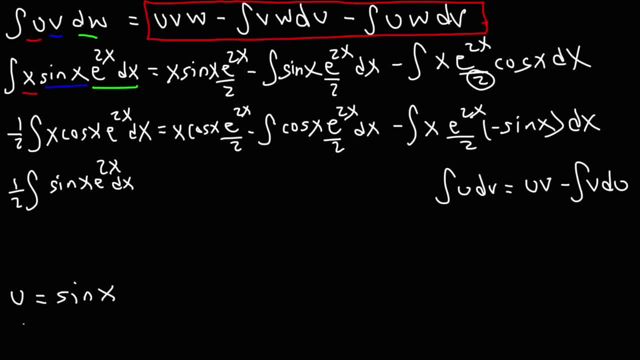 So u is going to be sine x, du is going to be the derivative of sine, which is cosine xdx. dv is going to be e to the 2xdx, And so v is e to the 2x over 2.. 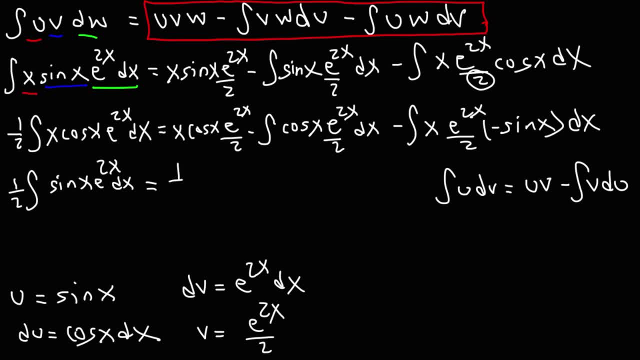 So this becomes u times v, So that's 1 half sine x. e to the 2x minus the integral of v du, So that's e to the 2x over 2 times du, which is cosine x dx. So notice that eventually we're going to be able to combine these two expressions. 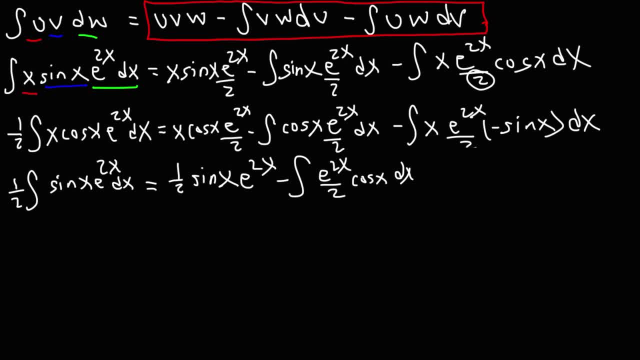 So at this point, what we want to do right now is take these terms and plug it in to their respective formulas. Now, one thing that we have yet to do is distribute the 1 half, So let's go ahead and do that now. 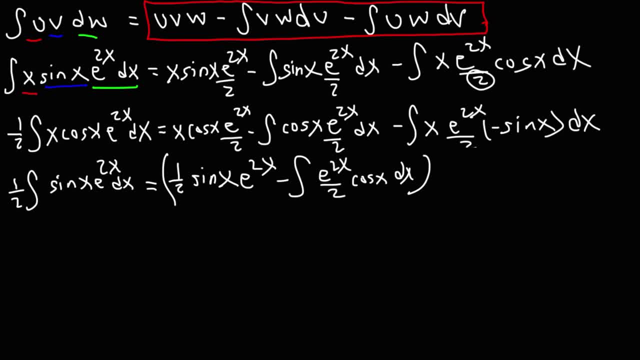 So, multiplying everything by a half, this becomes 1. fourth, And this becomes e to the 2x over 4.. Now we need to do the same with this expression. So let's replace all the twos with a four. So this would equate to dividing every term by 2, or multiplying it by a half. 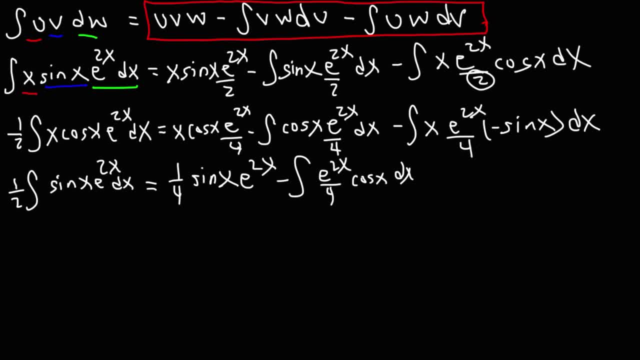 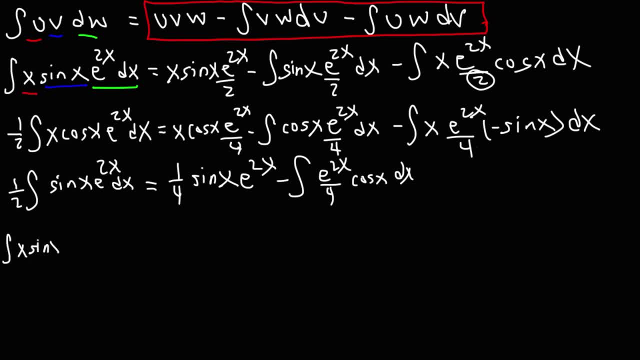 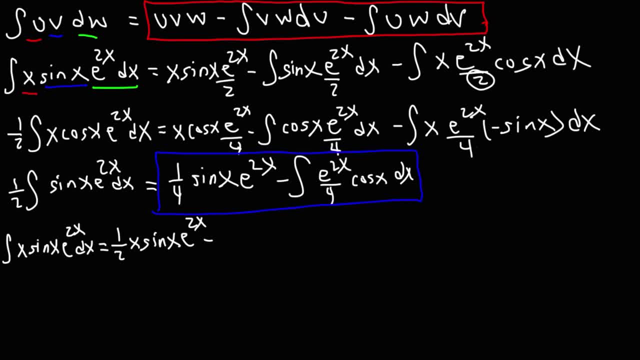 we see here it's going to be minus 1, 4th, sine x, e to the 2x and minus, minus that expression. so that's going to be plus 1, 4th, the integral of cosine x, e to the 2x, and let's not forget dx. so now we can move on. 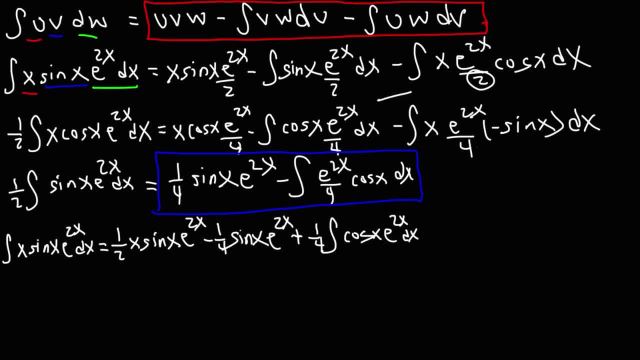 to this one, we do have a negative sign, so keep that in mind. so it's going to be minus. so we're going to replace this with everything that we see here. so it's minus that term. so that's going to be 1, 4th x, cosine e to the 2x, and then we 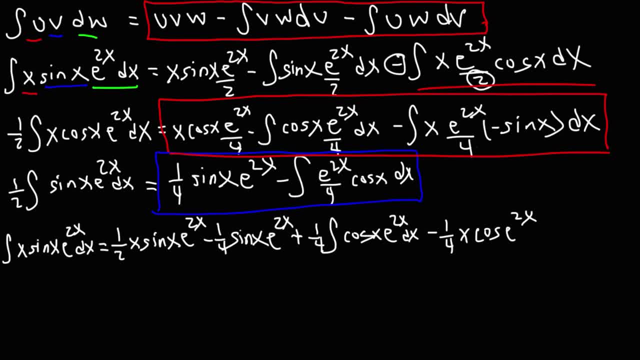 have minus and another minus, so that's going to be positive, which I'm going to put right under this expression because we can add them. so positive: 1, 4th, integral cosine x, e to the 2x, and then we have minus, minus, minus, three negatives. that's. 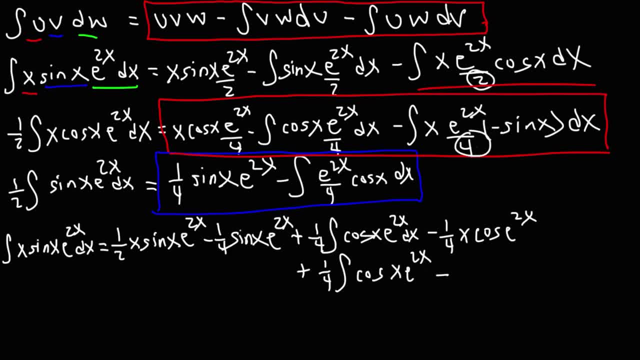 a negative. so minus. let's move the 4 to the front 1. 4th, the integral of x sine x e to the 2x dx. so what I'm going to do now is I'm going to take this and move it to the left side of the equation. so we have: 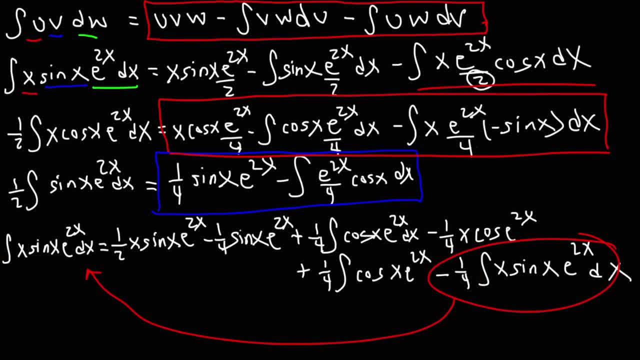 one plus 1 4th, that's four over 4 plus 1 over 4, which is five over four. so five over 4. integral x sine x e to the 2x dx is going to equal one half x sine x e to the 2x. so I'mus gonna take this and keep it to the left side of the equation. so we have 1 X sin xst, 6Dx, eigenient combo sin y sin 4x. 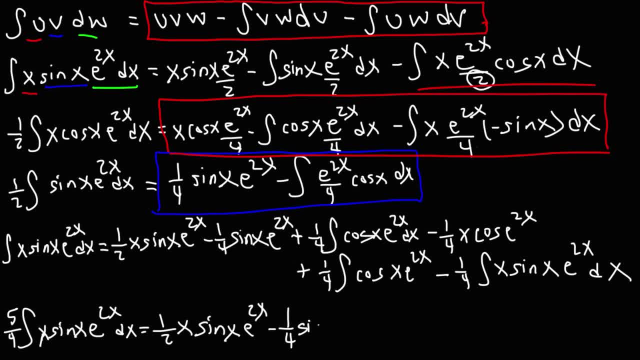 minus one-fourth sine x e to the 2x. One-fourth plus one-fourth is a half. so plus one-half integral cosine x e to the 2x dx, and then minus one-fourth x cosine x e to the 2x. 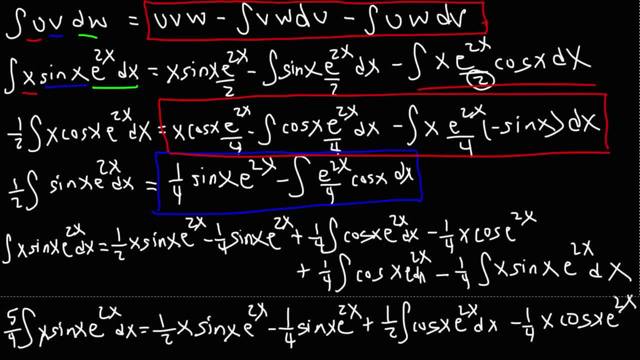 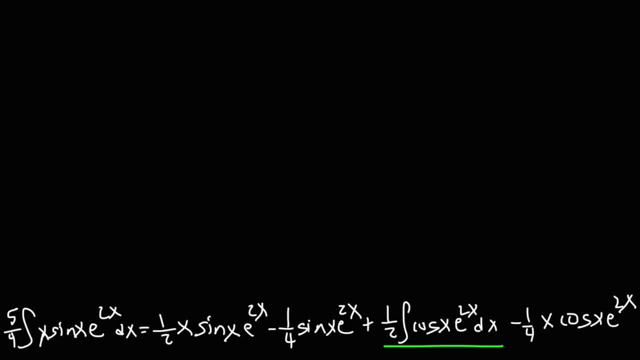 So now let's eliminate this and let's focus on this integral, The integral of cosine x e to the 2x dx. We'll deal with the one-half later. So we're going to make u equal to- let's put this on the bottom here. let's make u equal to cosine x. 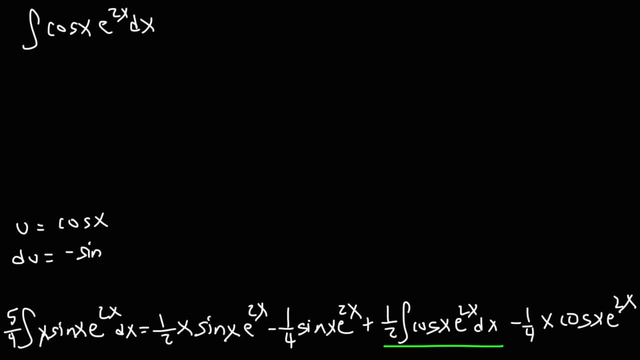 dx, So du will be negative sine x, dx and dv is e to the 2x dx, so v is going to be e to the 2x divided by 2.. So using the formula for a two-product term expression, it's going to be the integral of u, dv is u v minus the integral of v, du, So u times v. 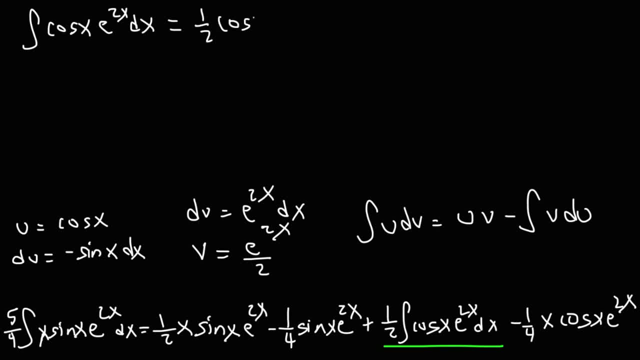 that's going to be 1.. One-half cosine x e to the 2x minus the integral of v du. So this is v, this is du. That's going to be negative sine x e to the 2x over 2 dx. So the two negative signs will cancel. 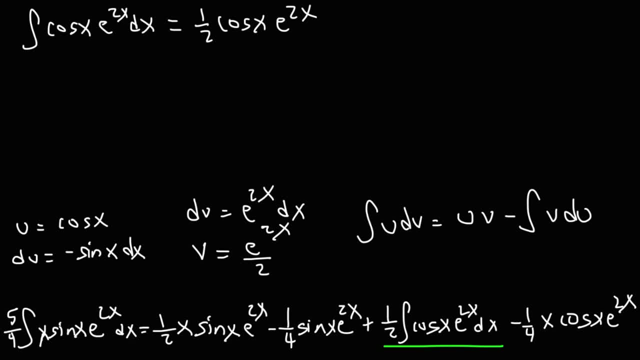 That's going to be positive and we can move the one-half to the front. So this becomes plus one-half the integral of sine x e to the 2x dx. Now we need to use integration by parts one more time. So this time we need to make u equal to sine x. du is going to be cosine x dx. 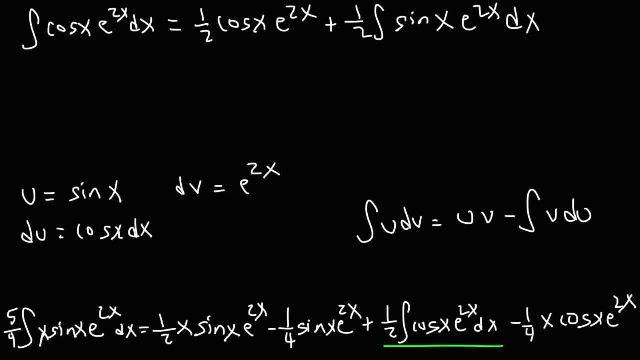 and dv is going to be the same. So this is equal to one-half cosine x, e to the 2x plus one-half. and now let's apply this formula, So it's u v, that's going to be one-half sine x e to the 2x minus the integral of v du, which is: one-half cosine x e to the 2x. So this is u v that's going to be one-half sine x e to the 2x, minus the integral of v du, which is one-half cosine x e to the 2x. 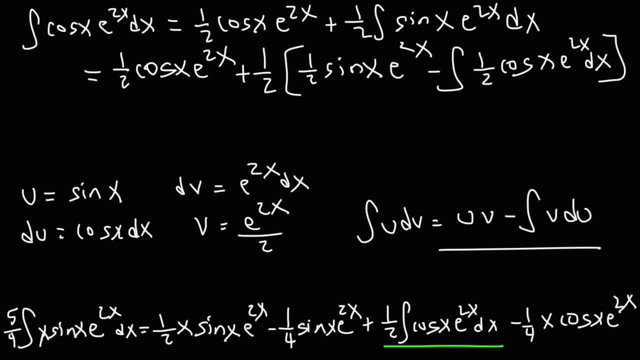 So this is u v that's going to be one-half sine x e to the 2x, minus the integral of v du, which is one-half sine x e to the 2x minus the integral of v du, which is one-half sine x e to the 2x. 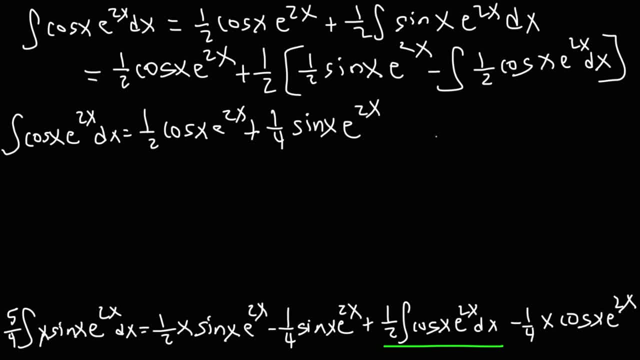 And then we have one-half times negative one-half. so that's negative one-fourth. integral cosine x, e to the 2x dx. So now we can combine these two expressions. So add in one-fourth integral cosine x, e to the 2x. this is going to be one plus one-fourth. 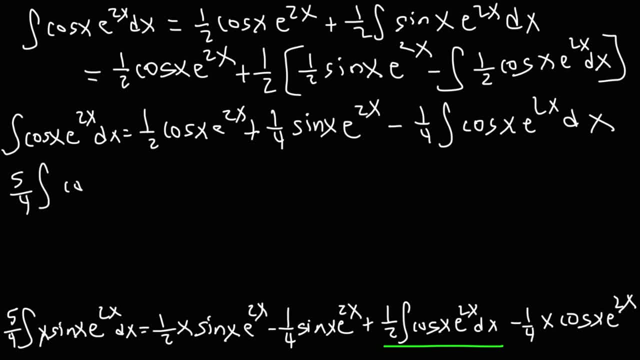 So we have five over four integral cosine x, e to the 2x, dx, which is equal to this. Now we're not trying to solve for five over four cosine x, e to the 2x. We want to find the value of. 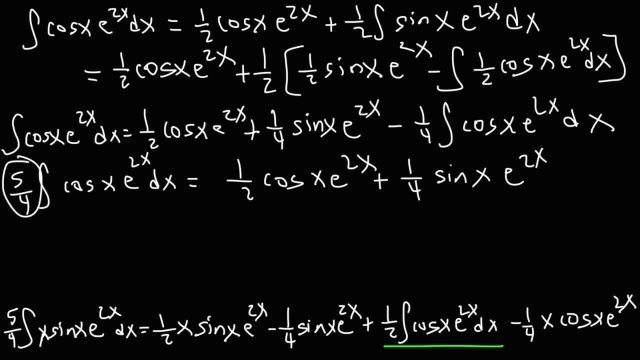 just one of it. So to turn this back into a one, we need to multiply everything by four over five, So the fours cancel, the fives cancel and we're going to get our original expression four over five times one over two. Four over two is two, so this becomes two over five. cosine x e to the 2x. Here the fours cancel, so that becomes one over five. sine x e to the 2x. 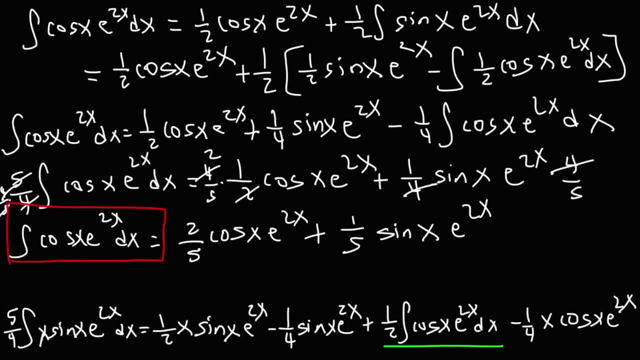 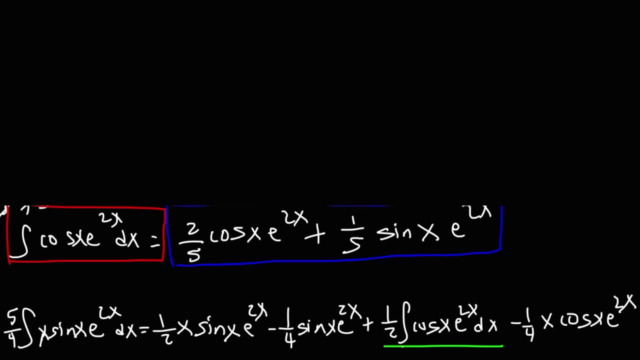 So the integral of cosine x e to the 2x is two over five cosine x e to the 2x plus one over five sine x e to the 2x. So we need to replace this expression with what we have here. 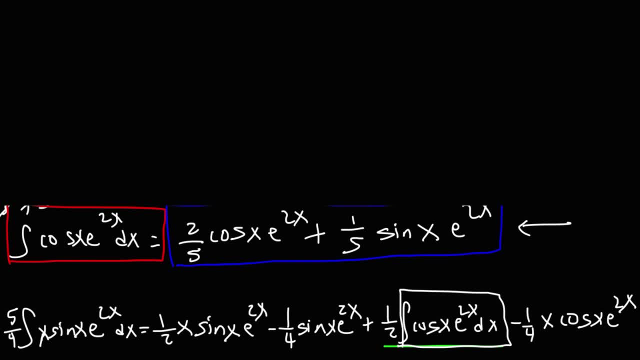 And then combine like terms, So five over four: integral x sine x e to the 2x dx, that's going to be one half x sine x e to the 2x minus one-fourth sine x e to the 2x. 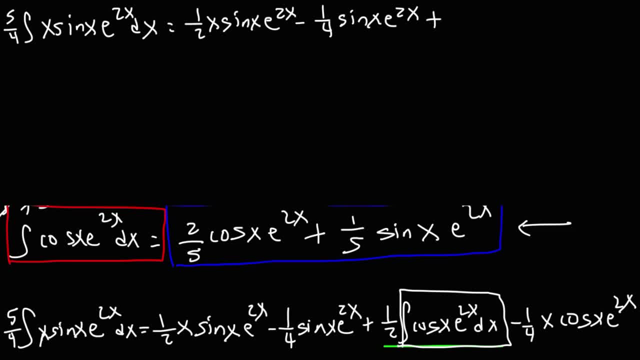 And then we have plus one half Times everything here, So times two over five: cosine x, e to the 2x, And then plus one half times this, That's times one over five: sine x, e to the 2x, And then 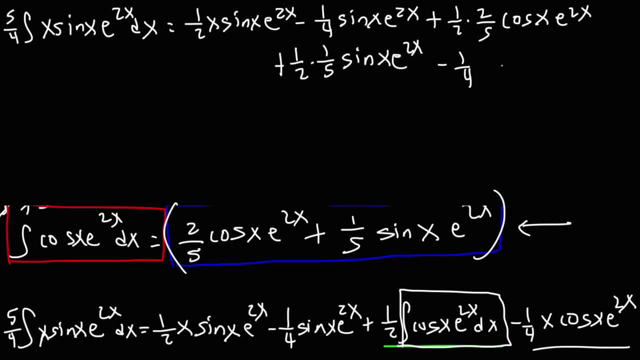 That one Minus one-fourth x, cosine x, e to the 2x, So we can combine those expressions. So that is negative. one-fourth plus This is one over ten, So again common denominator, so we need to get to 20.. 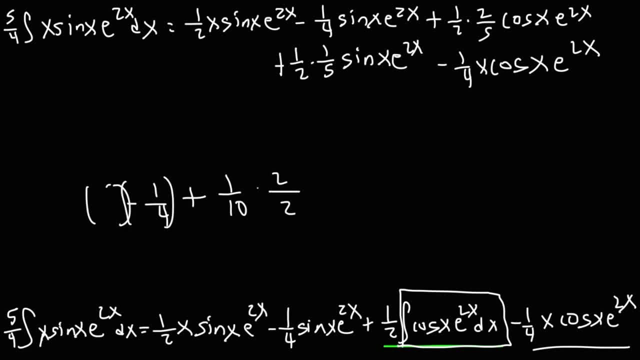 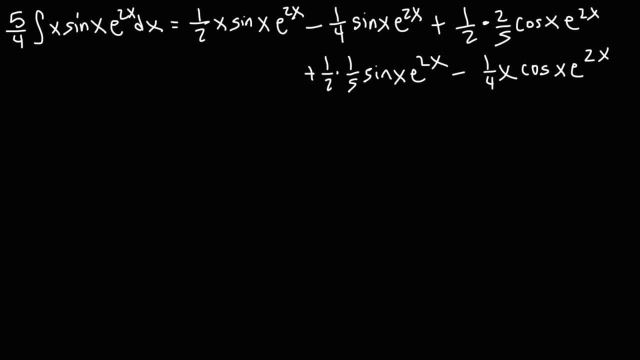 We're going to multiply that by two over two And this by five over five, So we get negative five over 20 plus two over 20, which becomes negative three over 20.. In case you're wondering why the screen looks a little different, there's no cause for concern. 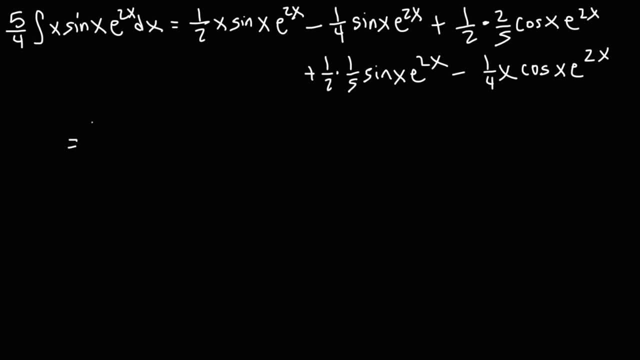 I just had to do some video editing, So we're going to do some video editing, So let's put everything together at this point. So these expressions combined, We said it's negative three over 20 sine x. e to the 2x. 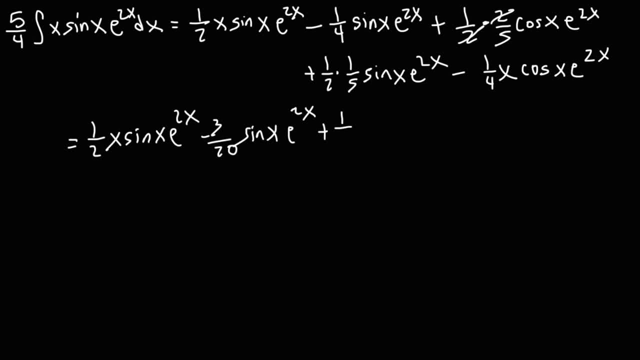 And then these will cancel. So we're going to get plus one over five, cosine x e to the 2x, And then minus one-fourth x, cosine x e to the 2x. Now we need to replace the five over four with a one. 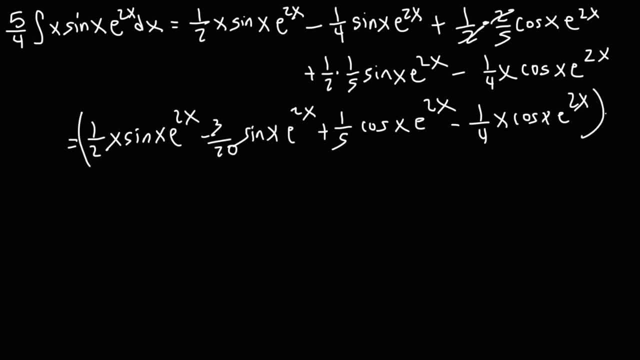 So we're going to multiply every expression by four over five. So the fours will cancel, The fives will cancel. On the left, we're going to get the integral of x sine x, e to the 2x. These will cancel. 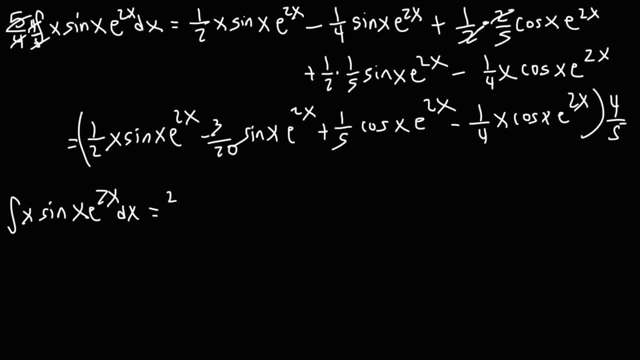 Four divided by two is two, So this will give us two over five, x, sine x, e to the 2x, Three over 20 times four over five. That requires some work. Twenty can be written as four over five, And so we can cancel the four, which will give us three over 25.. 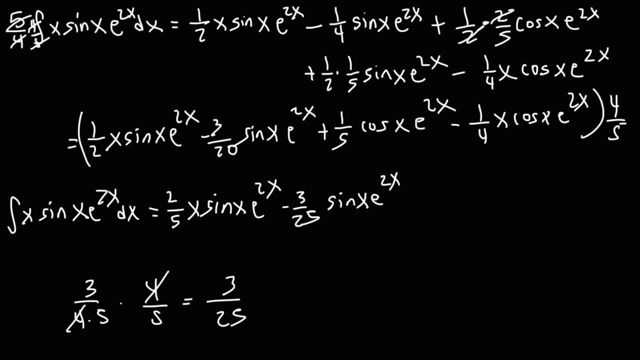 And then we can multiply these two: Four over five times one over five, That's going to be four over 25. cosine x e to the 2x, And then these will cancel giving us negative one over five x. cosine x e to the 2x plus c. 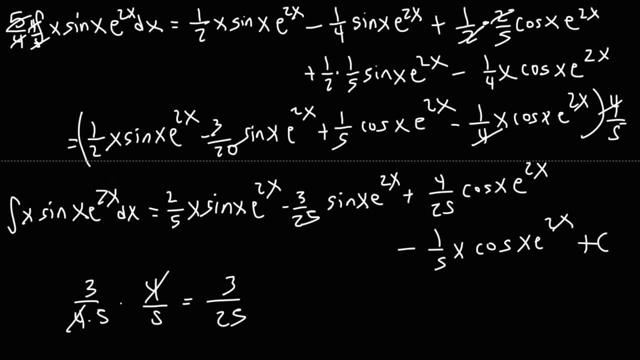 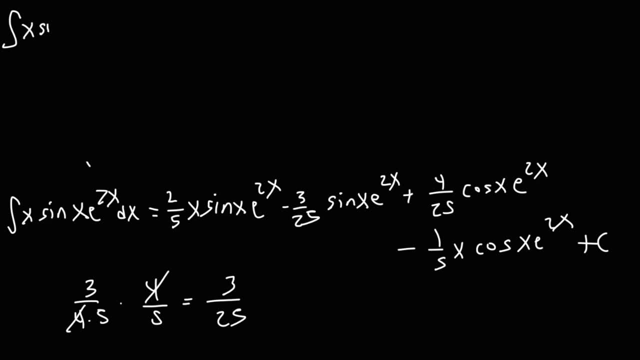 So we're going to get four over five x sine x e to the 2x, And then these will cancel giving us negative one over five x cosine x e to the 2x plus c. So thus we have our final answer, which I'm going to write on the top of the screen because we're going to check our work soon. 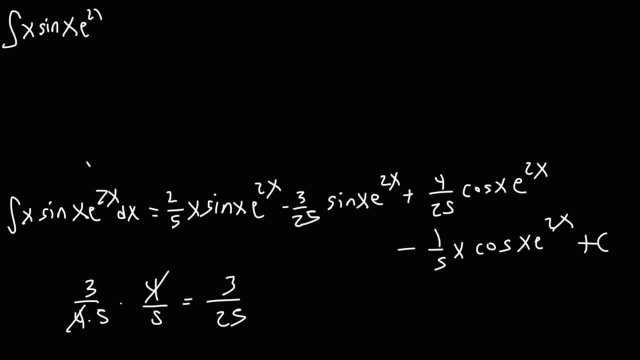 So the integral of x sine x e to the 2x dx is equal to two over five x sine x e to the 2x, And then minus three over 25 sine x e to the 2x, And then minus three over 25 sine x e to the 2x. 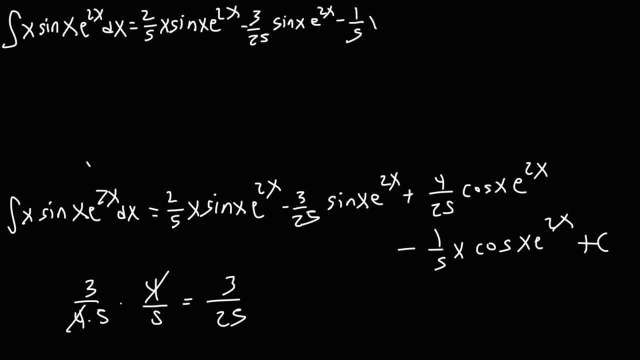 E to the 2x, minus one over five x. cosine x e to the 2x, And then plus four over 25: cosine x e to the 2x plus c. So this is the final answer. So that's how you could find the indefinite integral of a three product term expression using integration by parts. 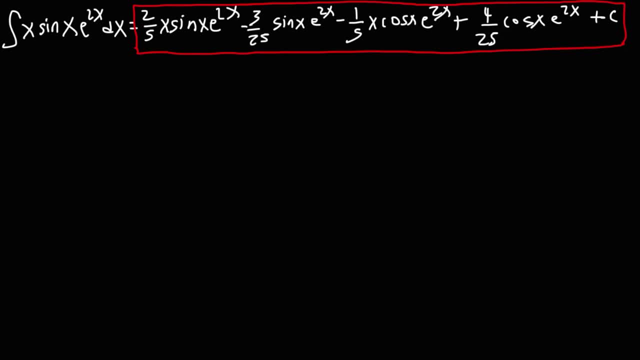 Now, in order to make sure that this answer is indeed correct, we're going to take the derivative of the right side of the equation and make sure we get what is on the left side. So let's take the derivative of the first term, two over five, x sine x, e to the 2x. 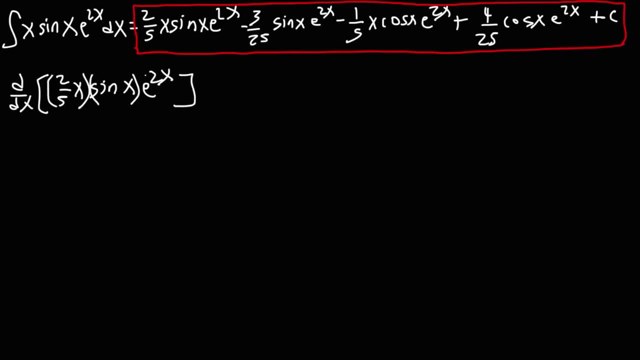 So we're going to use the product rule, given this three term expression. First we're going to differentiate the first part, two over five, x, The derivative of x, is one, so it's two over five times one. And then we're just going to multiply by the other two products sine x, e to the 2x. 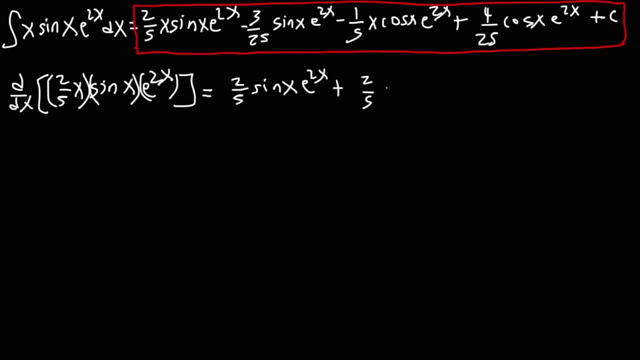 Next, we're going to leave the first part the same. We're going to take the derivative of the second part- The derivative of sine is cosine- and we're going to leave the third part the same. For the last one, we're going to differentiate the third part, which is e, to the 2x times two. 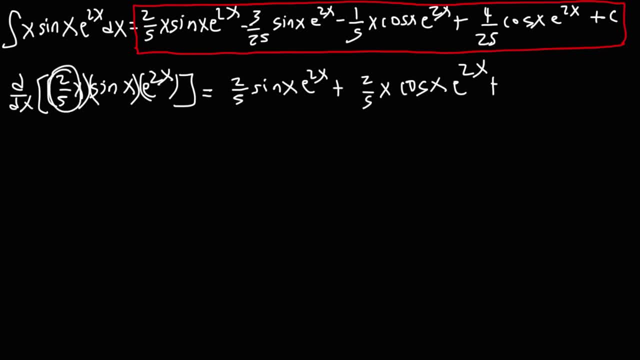 We're leaving these two the same, So two times this will be four over five, x, sine x, and then e to the 2x. Now let's take the derivative of the next term, that is, of negative three over 25, sine x, e to the 2x. 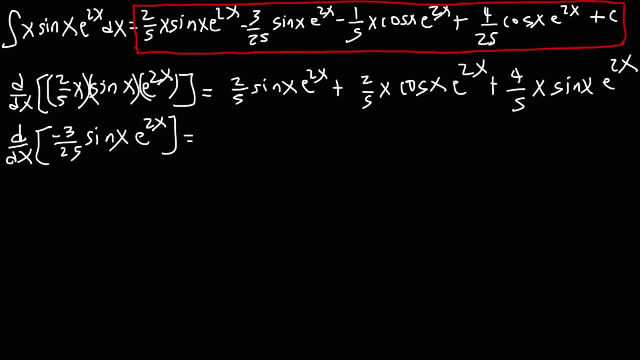 So we need to use the product rule again, but for a two product term expression. Let's say: this is u, this is v. So the derivative of the first part is going to be negative three over 25 times the derivative of sine, which is cosine. 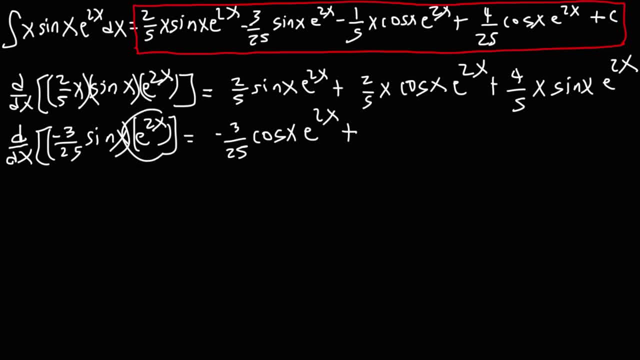 We're going to leave the second part the same. Next, we need to differentiate this part: e to the 2x, which is just e to the 2x times two, So negative three over 25 times two. That's going to be negative six over 25, sine x: e to the 2x. 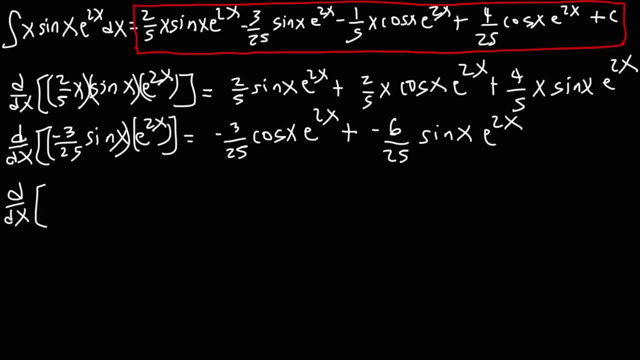 Now moving on to the next term. The next one is going to be negative one over 5 x. cosine x e to the 2x. So we have a three product term expression. The derivative of negative one over 5 x is just negative one over 5.. 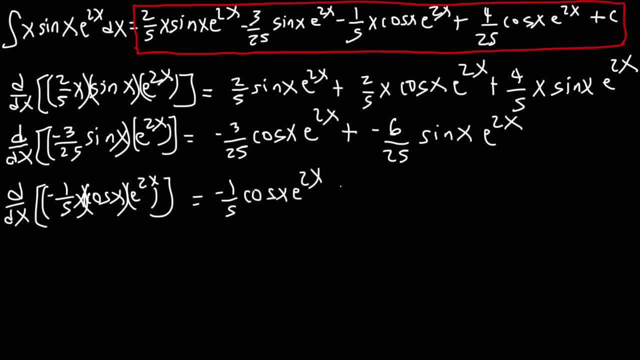 And then we're going to have cosine times 2x, times e to the 2x. The derivative of cosine is negative sine, so this is going to be positive 1 over 5x. sine x, e to the 2x And the derivative of e to the 2x is the same thing times 2,. 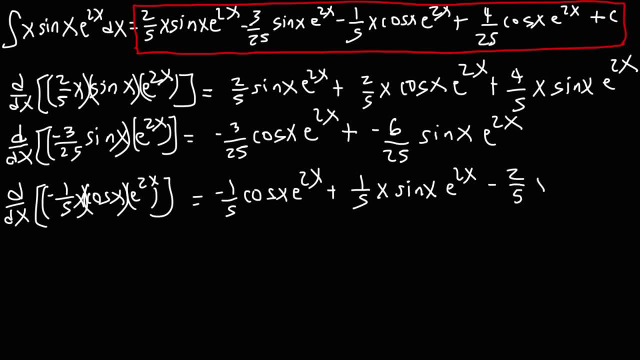 so it's going to be negative 2 over 5x. cosine x e to the 2x. Now for the last one: 4 over 25. cosine x e to the 2x. we have a two-product term expression. The derivative of cosine is negative sine. so we're going to have negative 4 over 25. 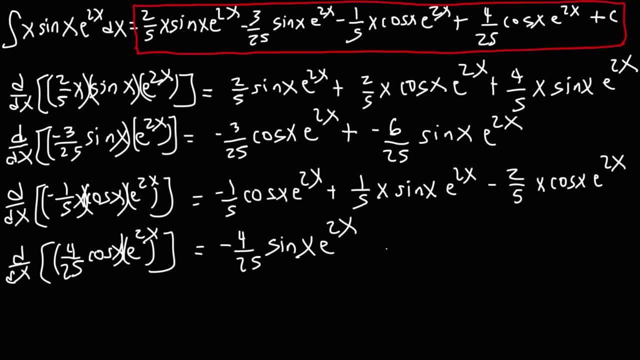 sine x, e to the 2x, And then the derivative of e to the 2x is going to be that times 2, so 4 times 2, that will be 8.. And then the derivative of cosine is negative: 2 over 5x. sine x, e to the 2x. 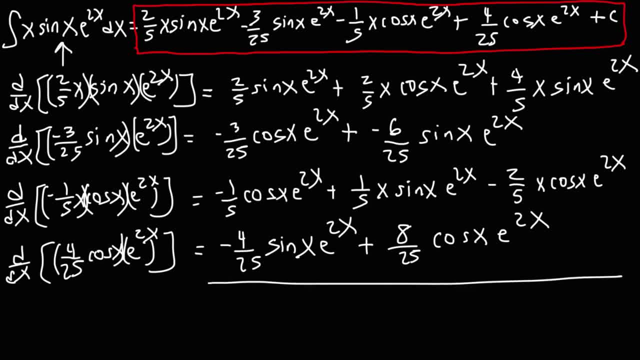 What we're going to do is add these terms and see if we get this. Let's think about what cancels These two terms cancel. Let's see what else. Let's focus on D-stream. d stream negative 3 over 25. negative 1 over 5. if you multiply that by 5 over 5. 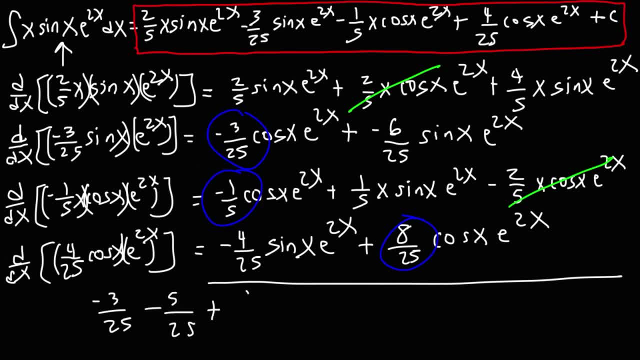 you get negative 5 over 25 plus 8 over 25. that adds to 0. so therefore we can cancel these three terms. now let's talk about these numbers here: 2 over 5. multiplying that by 5 over 5, that's going to give us 10 over 25, and then we have 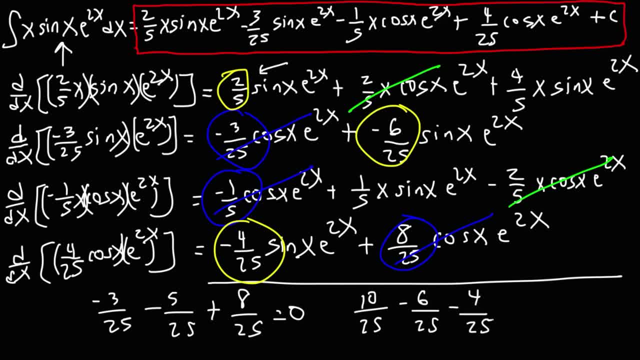 minus 6 over 25 minus 4 over 25. that's going to give us 0 as well, so we could cancel these those three terms. so what we have left over is the negative 3 over 5 minus 6 over 25. minus 4 over 25 minus 4 over 25 minus 4 over 25. 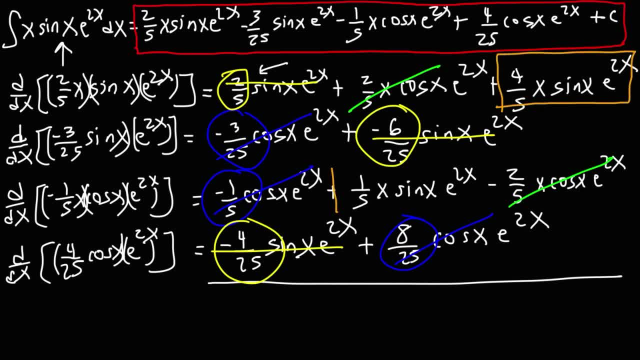 is the sum of these two, 4 over 5 plus 1 over 5, is 5 over 5, which is just 1. so we get 1 x sine x, e to the 2x, which is our original expression. so therefore, this is indeed the correct answer. so that is.